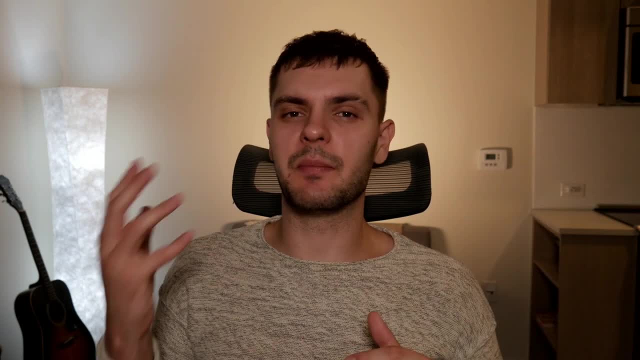 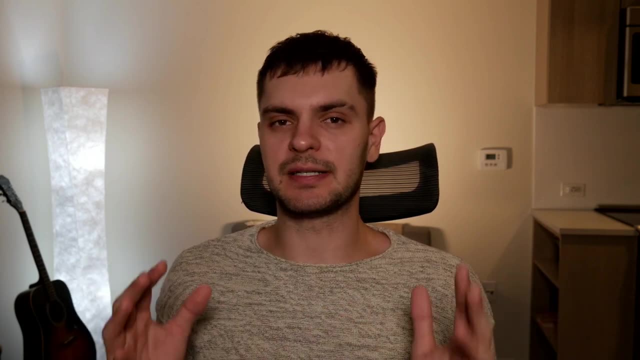 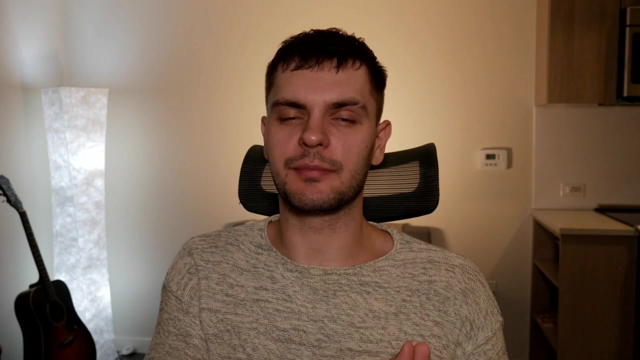 Objects are made out of data and methods that operate on that data. In Rust, structs and enums hold data and you can use implementation blocks to provide methods on structs and enums. So, even though structs and enums are not called objects, they provide the same functionality. The next: 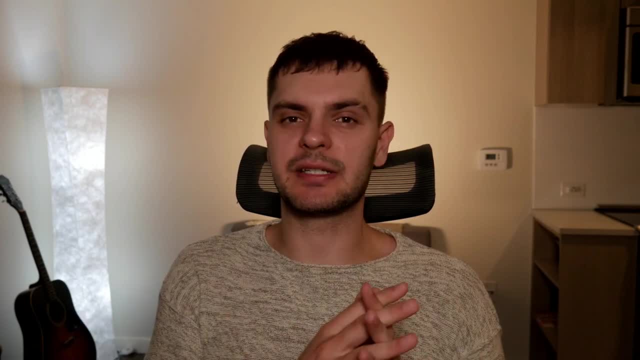 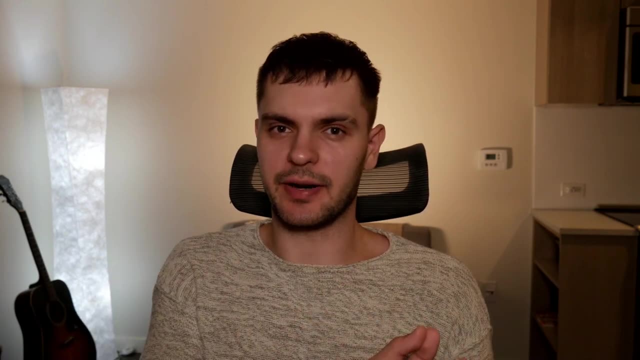 characteristic is encapsulation, which means that implementation details of an object are hidden from the code using that object. Instead of changing the structure of an object, you can change the internals directly. Code outside of the object is limited to interacting with the object through its 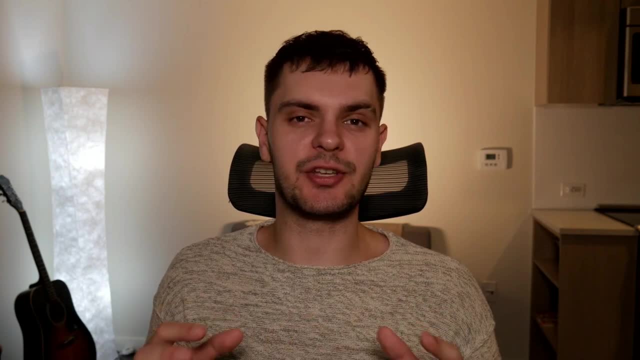 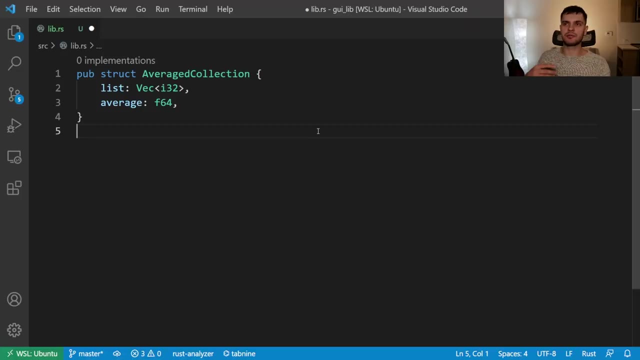 public API. This enables the programmer to change the internals of an object without changing code which uses that object. In chapter 7, we learned how to use the pub keyword to decide which modules, types, functions and methods are public, because in Rust everything is private by default, For example: 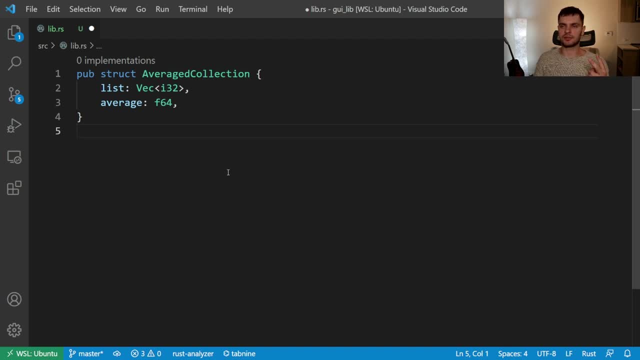 here we have a struct called averagedCollection. It contains the object's name and the object's name. It contains two fields: a list of integers and the average of those integers. Here our struct is caching the average such that it doesn't have to be computed on demand every time. Notice that. 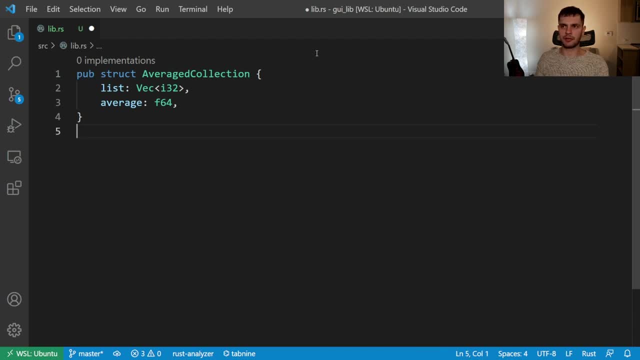 our struct is public, so that code outside of this library can use our struct, but the fields are private, And this is important in this particular case, because we want to make sure that when this list is updated, when elements are removed or added, the average is also updated Instead of 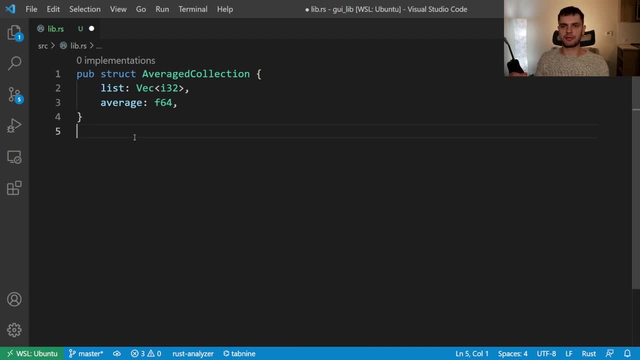 letting code manipulate the structure of an object. we want to make sure that the object is in the same state as the object. In order to manipulate these internals directly, we're going to create an implementation block with methods that modify the internal state. Here we have an. 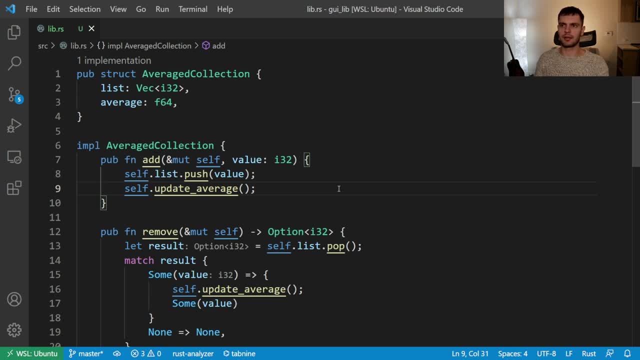 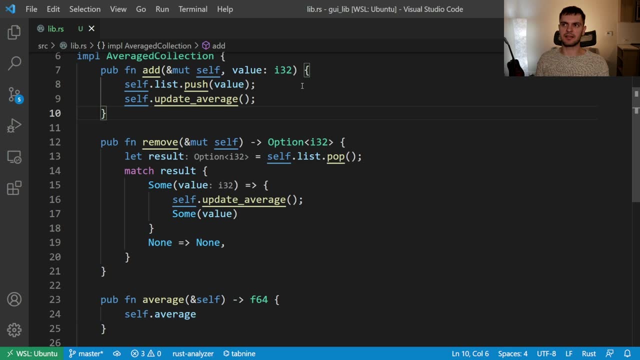 implementation block for our averagedCollection struct. It has three key methods: add, remove and average. The add method takes a mutable reference to self and a value. Then it adds that value to the list and calls updateAverage. The remove method takes a mutable reference to self. 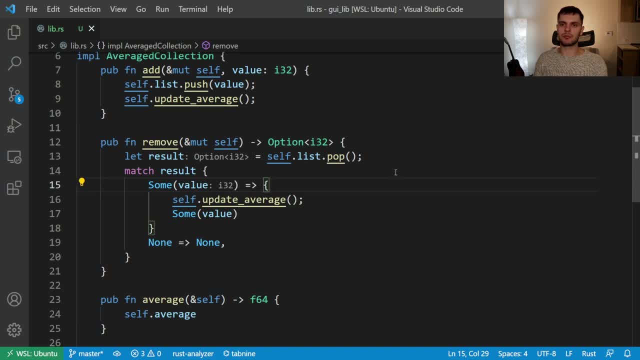 and returns an optional integer. In this case we want to make sure that the object is in the same state inside the method. The first thing we do is call popOnThatList, which will remove a value, And this will return an optional integer which we store in result And then we match on result. 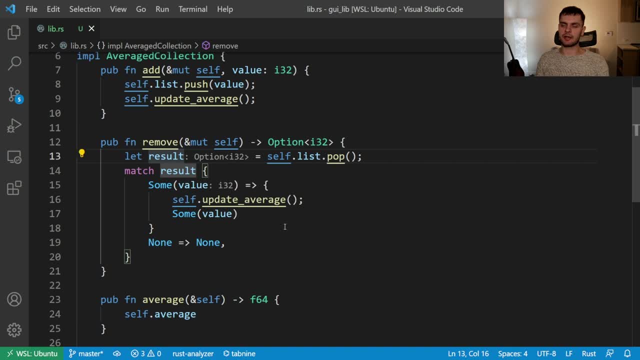 If we get a value, then we update average and return that value, And if we get none, then we simply return none. We also have a method called average, which takes a reference to self and returns a 64 bit floating point number. Here we simply return a self dot average. we don't have 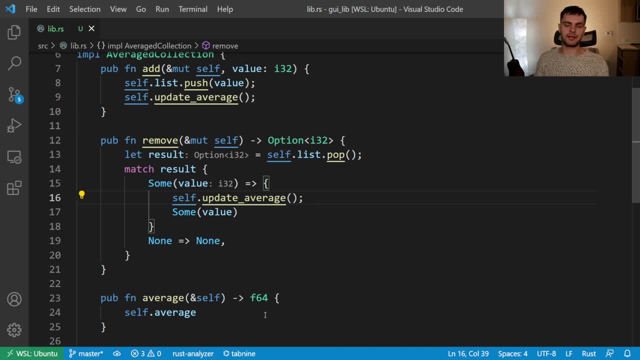 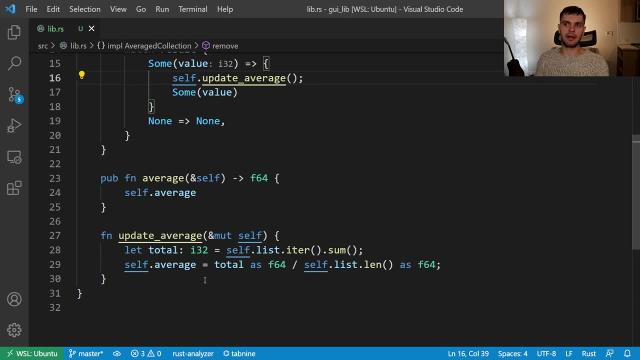 any extra calculations in this method, because our two methods that modify the list- add and remove- call updateAverage And if we scroll down you'll see we have a private method called updateAverage. updateAverage will take a mutable reference to self calculate the average and then store that. 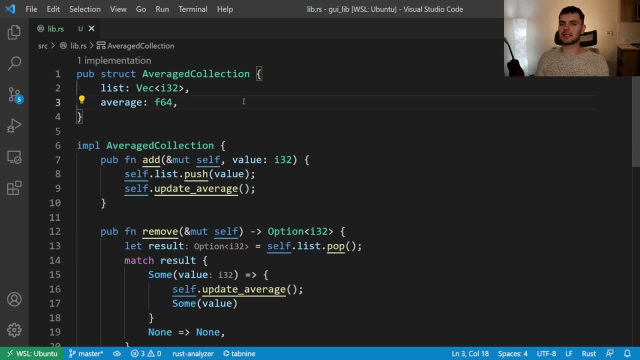 inside self dot average. Because we've encapsulated the internals of averagedCollection, we could change the internals without changing code that uses our struct. For example, instead of storing our integers in a vector, we could store them in a hash set. Then the methods to 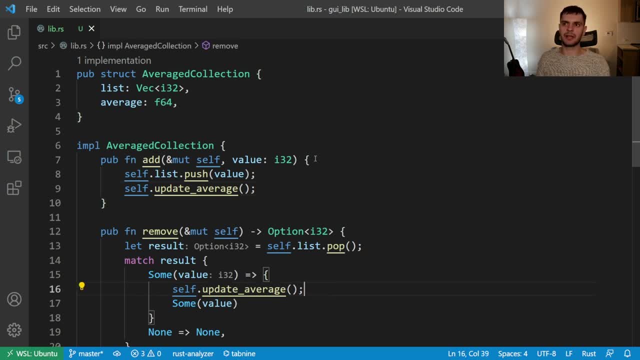 add and remove numbers from that hash set will change. But as long as our public add and remove functions have the same signature code using our struct, doesn't have to care. So to summarize the fact that things are private by default, but you can use the pub keyword to make things public. 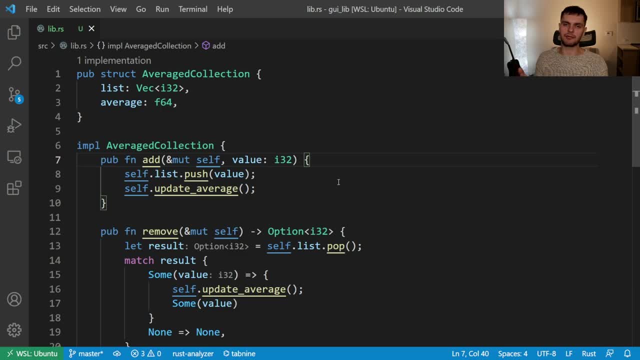 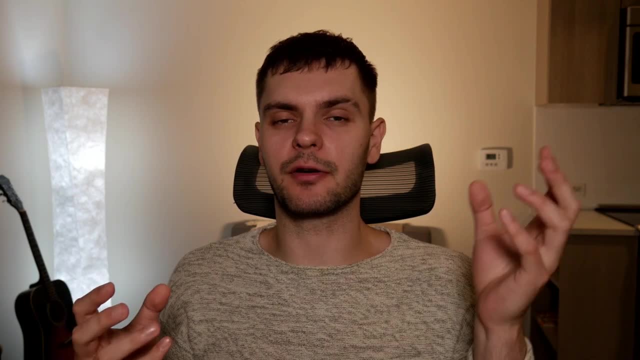 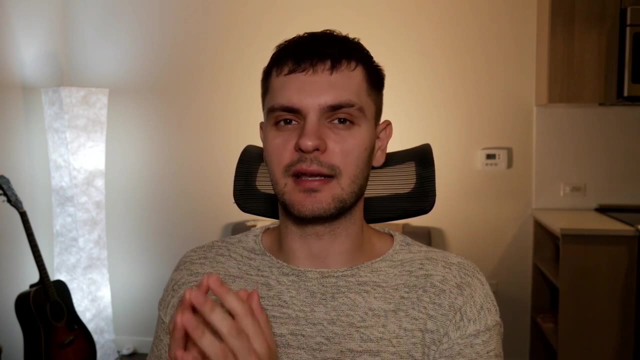 gives you the ability to encapsulate implementation details in Rust. Finally, let's talk about inheritance. Inheritance is the ability for an object to inherit from another object's definition, gaining the data and behavior of that other object without having to define the data and behavior. 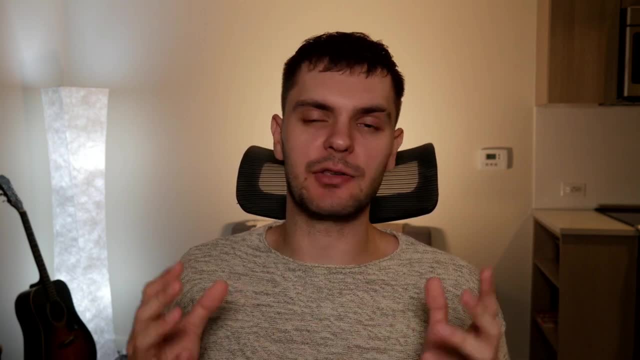 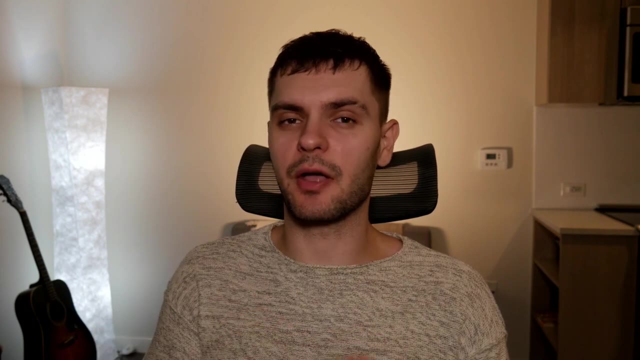 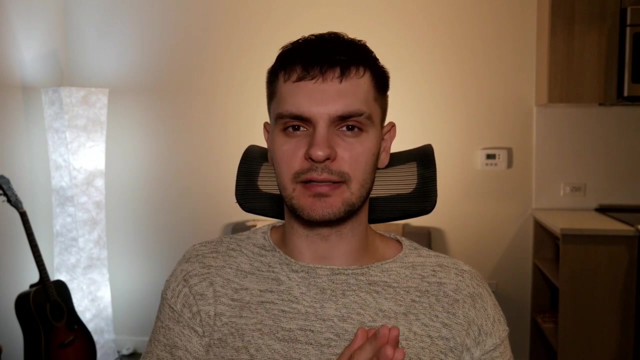 itself. Rust does not have this ability. Specifically, you can't define a struct that inherits fields and methods from another struct. Rust, however, does have some other tools you can use, depending on why you're reaching for inheritance. There are two main reasons for using. 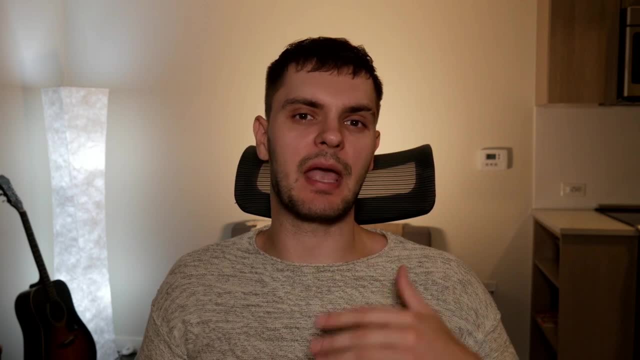 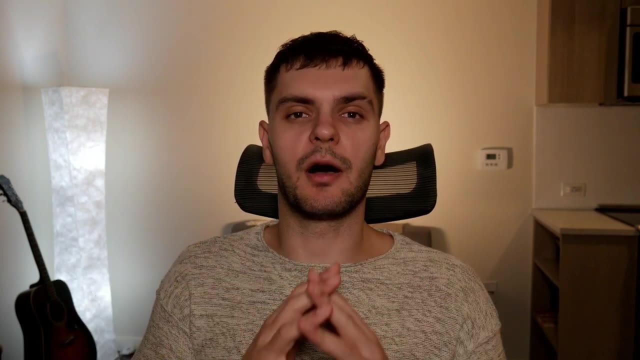 inheritance. The first one is code sharing. You can implement behavior on one type and then all the other types that inherit from it can reuse that behavior. In Rust, you can accomplish the same thing by using default trait method implementations. Note that there is a limitation. 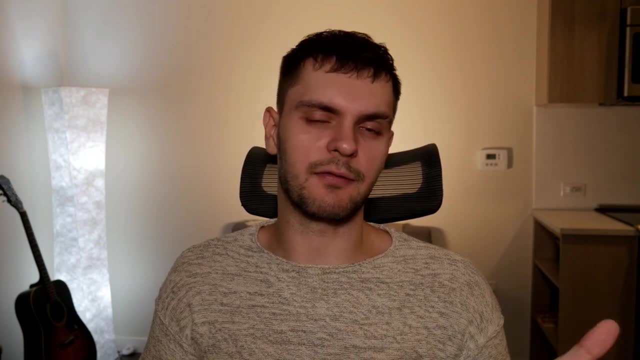 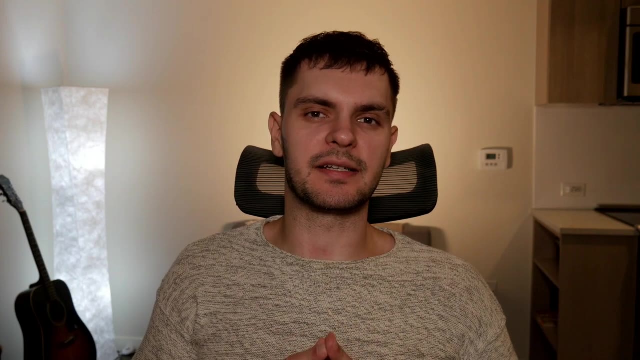 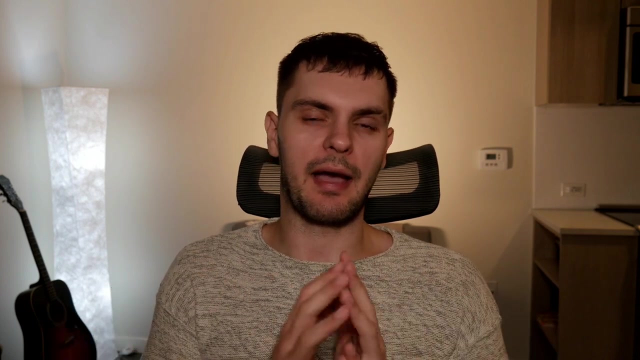 As of this video, traits can only define methods, not fields, although there is a proposal out there that will allow traits to define fields. The other reason to use inheritance is for polymorphism. Polymorphism allows you to substitute multiple objects for each other at runtime if they share.